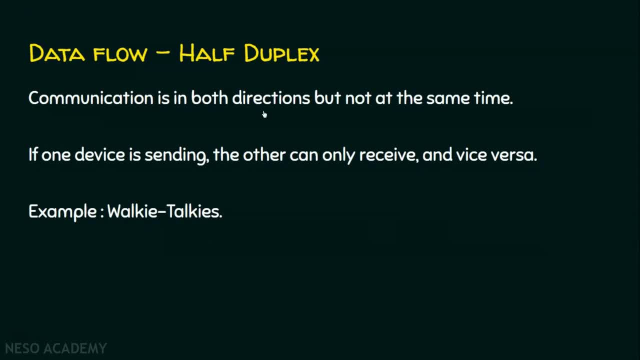 Coming to the half duplex, the communication is in both directions. It means, it can send as well as it can receive, but not at the same time. 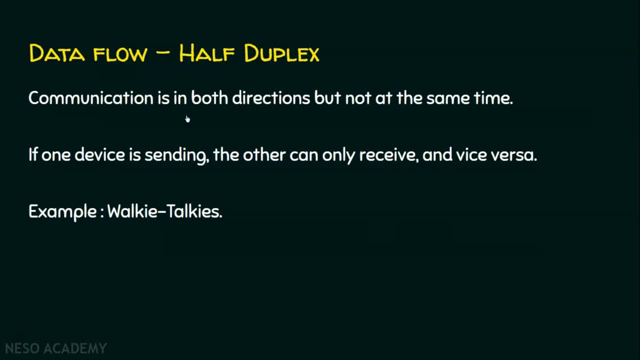 The very important part about half duplex is that, the communication can happen in both directions, but not at the same time. If one device is sending, the other device can receive. And not at the same time, both sending and receiving can happen. Example walkie-talkie. In a walkie-talkie, we can talk as well as we can listen, but we can't talk and listen at the same time. 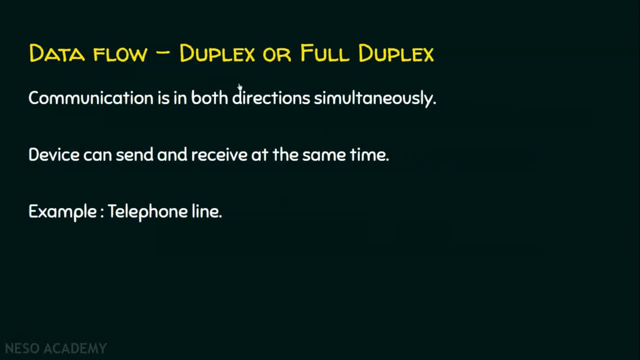 Now we shall see what is full duplex or simply duplex. 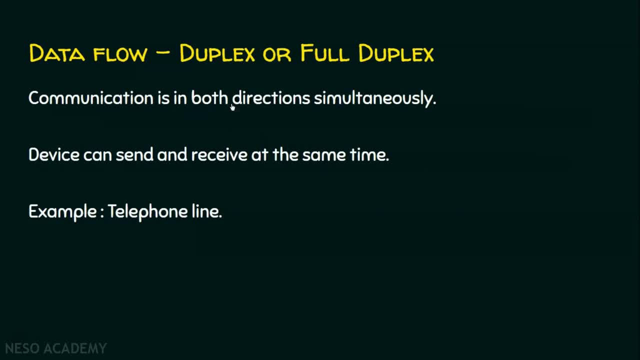 In the previous case, that is the half duplex, communication happened in both directions, but not at the same time. 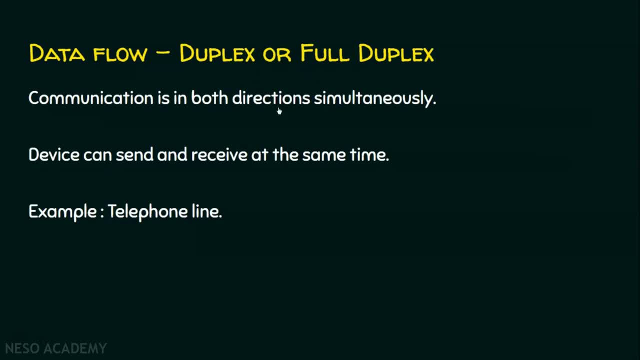 Whereas in full duplex, communication can happen in both directions simultaneously. 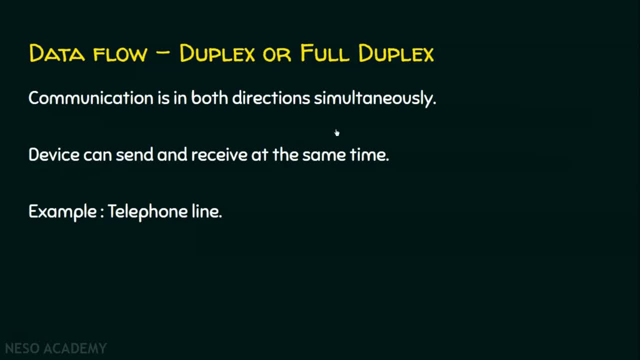 It means, devices can send or receive data at the same time. Example telephone line. 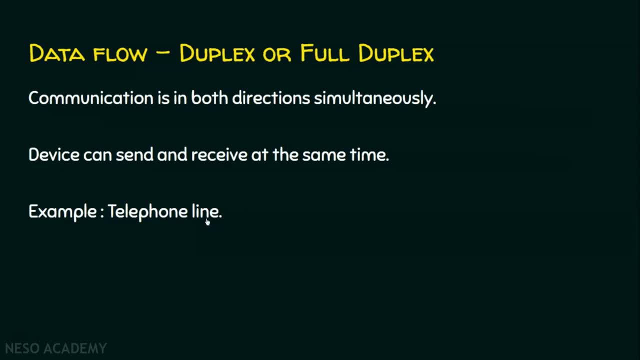 We can talk as well as listen simultaneously in a telephone line. Now we shall see an example for simplex communication. 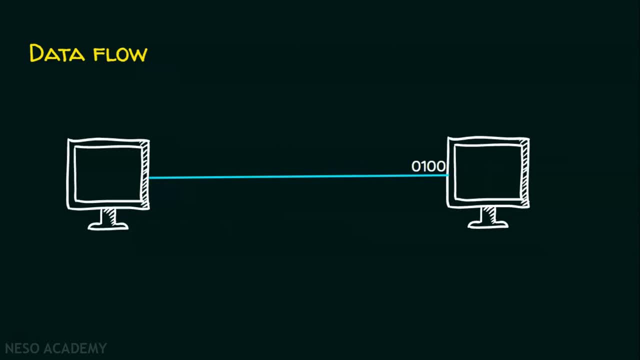 Now this computer is sending data in only one direction. So this is simplex. 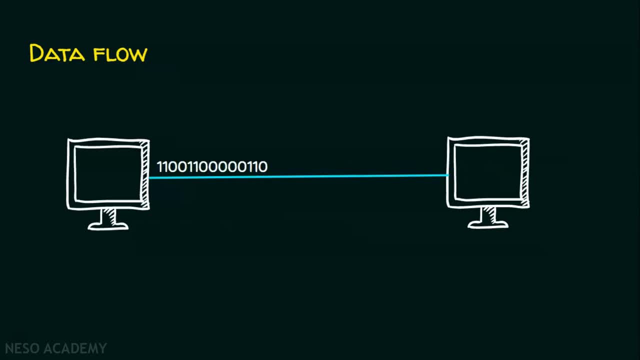 If both sending and receiving can happen, but not at the same time, if you observe, now sending is happening, now receiving is happening, but not at the same time. This is sending and this is receiving. This is not happening at the same time. 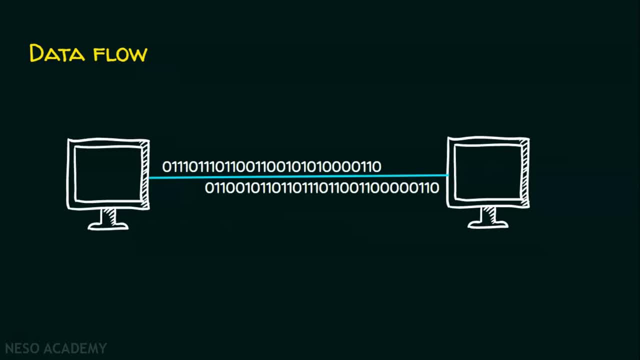 So this comes under half duplex. In full duplex mode of communication, both sending and receiving can happen at the same time. 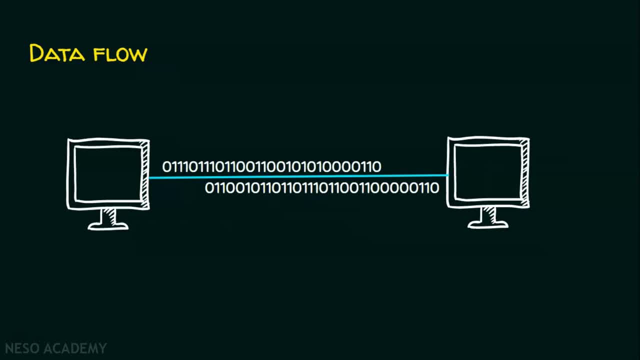 If both sending and receiving can happen simultaneously, then we call as full duplex. 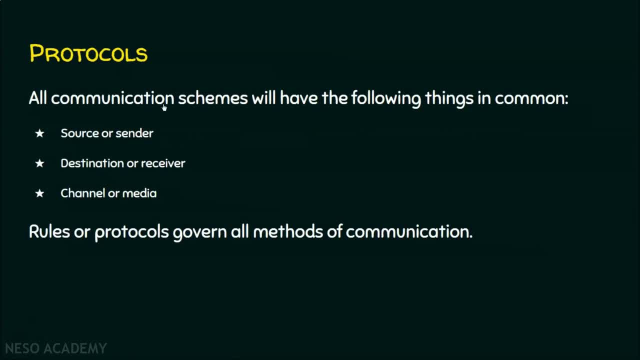 We will now see what are protocols. Any communication scheme. Whether it is a postal communication or a WhatsApp communication or SMS way of communication, we always have certain things in common. 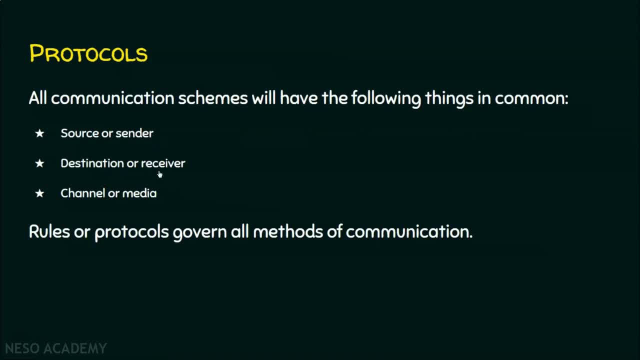 They are source or sender, destination or the receiver, channel or media. Any communication will definitely have these things. 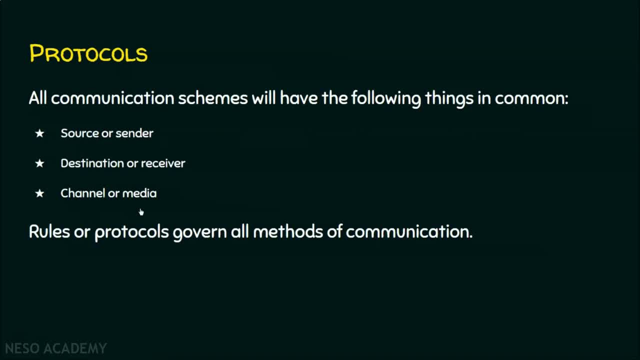 Source or the sender, destination or the receiver, channel or the media. 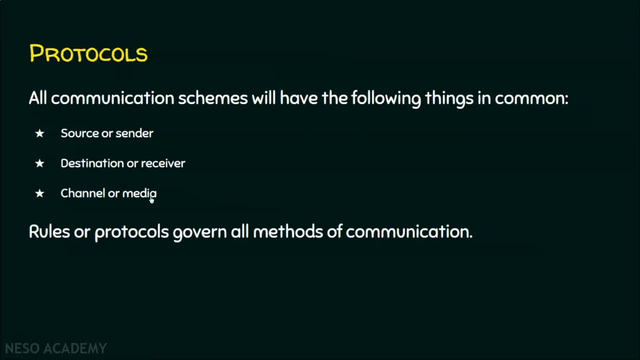 And this communication will always be governed by certain protocols. So protocols are rules that governs all the media, methods of communication. 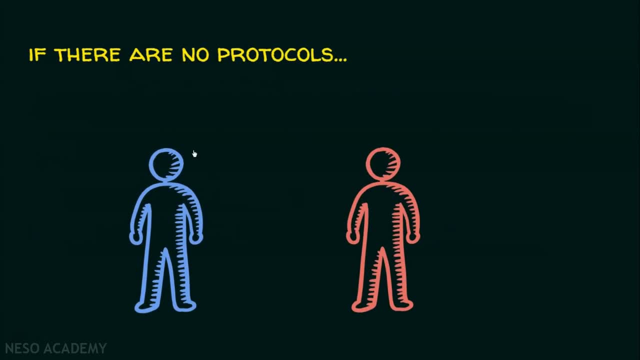 What if there are no protocols? If this guy speaks at high speed, which this destination cannot handle, this communication becomes useless. 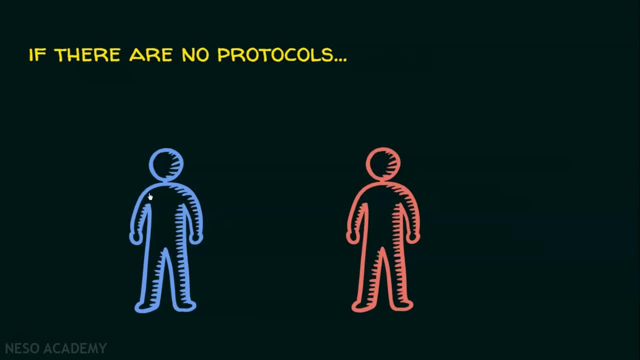 So they have to mutually agree upon certain rules. What if this blue guy speaks in the language which this guy cannot understand? He may be grammatically correct, but still there is no use in this communication. 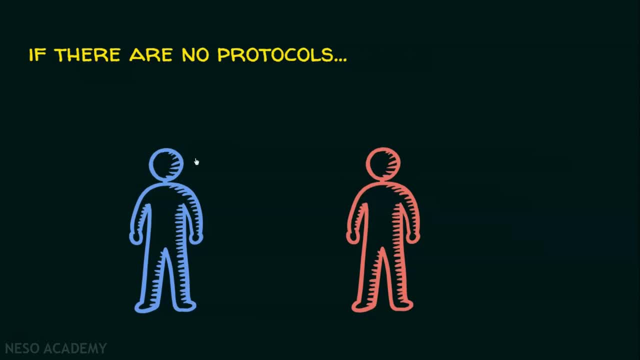 Again, what if this blue guy keeps on talking at a high speed at the same time not at all giving any room for this guy to respond? 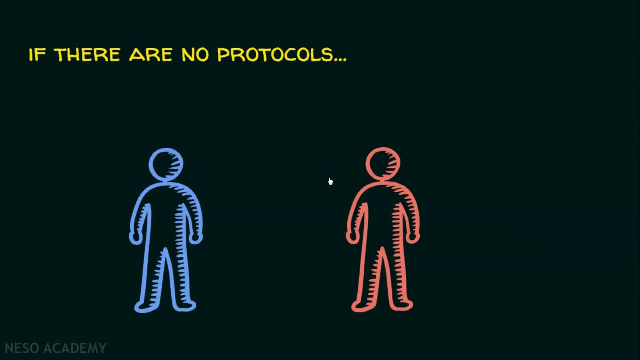 So these are example situations where the communication goes kiosk or messy. 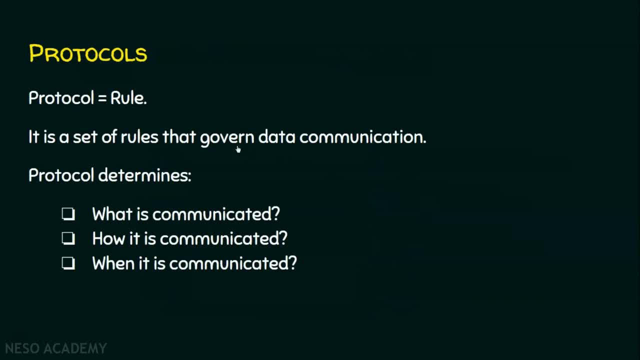 So definitely there is a need for protocols. Because a protocol is a set of rules that governs data communication. Simply speaking, protocol is a rule that governs data communication. 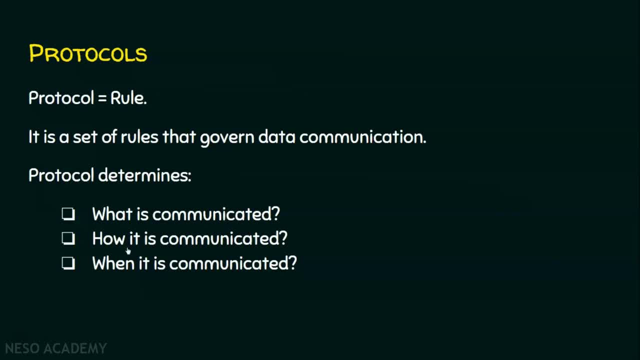 Protocol determines what is communicated in the network, how it is communicated in the network and when it is communicated. 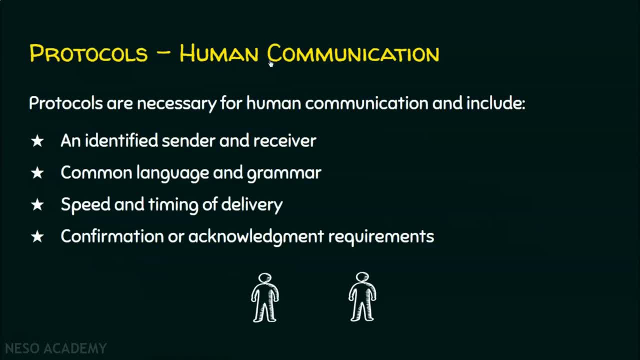 Before going into the network communication, let's talk about the protocols in the human communication. 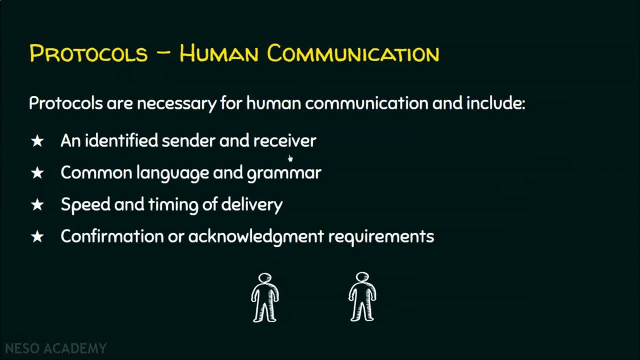 In human communication, definitely there should be sender and a receiver. There may be a single receiver or a group of receivers. And this human communication can be effective only when this communication involves common language and grammar. 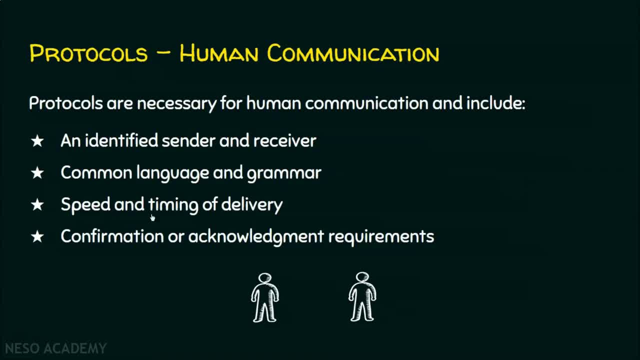 Otherwise, communication will not be perfect. And speed and timing of delivery of speech is also very important in human communication. 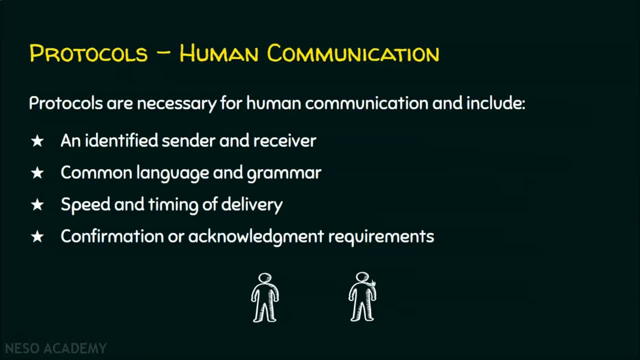 And if this guy wants to ensure whatever he has talked is understandable by this guy, he should get confirmation or the acknowledgement from the receiver, that is the destination. Only then human communication can be effective. We have just seen what is human communication. Why do we need protocols in human communication? Now we shall see why do we need protocols in network communication. 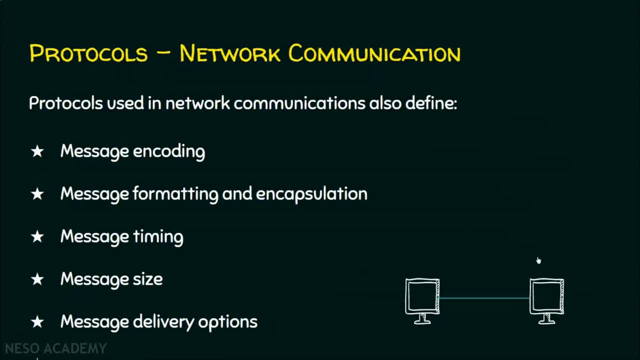 Say if there is a sender and there is a receiver and this communication can be effective when these protocols are addressed properly. The message should be encoded formatted and encapsulated in such a way that the destination can understand. 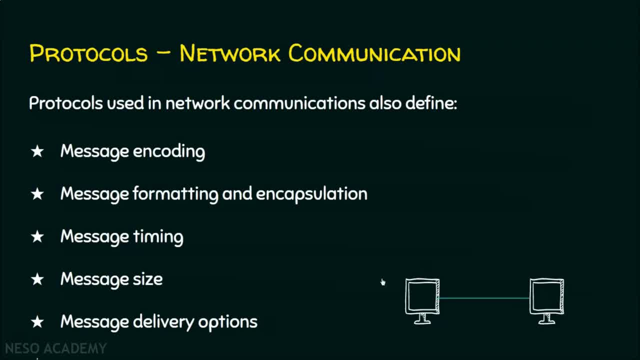 Timing is also very important in network communication. The size is also very important because the link cannot carry big data. If this is a low capacity link, then this link cannot carry big data. If there is a very big data in the sender side, it cannot send that big data on a very small link. So it has to be handled appropriately. At the same time, the delivery option should also be dealt. 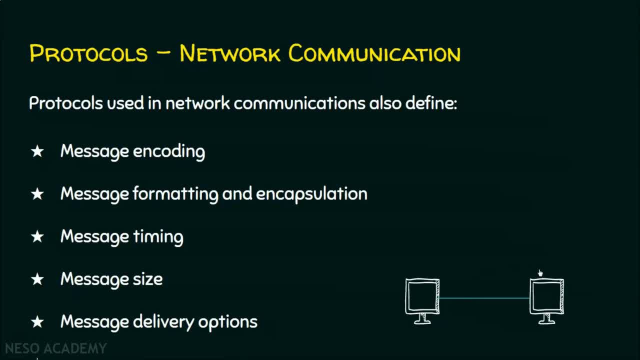 Whether the message is only for one destination or some group of destination or all the destinations in the network. 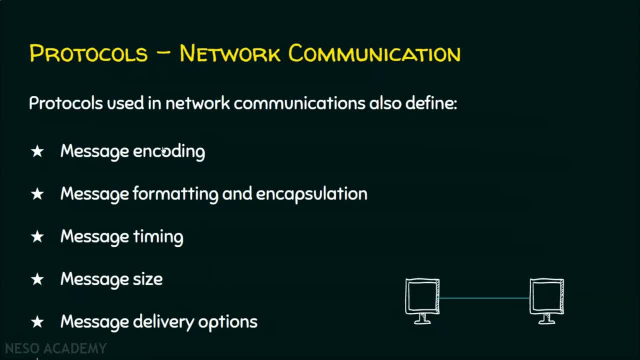 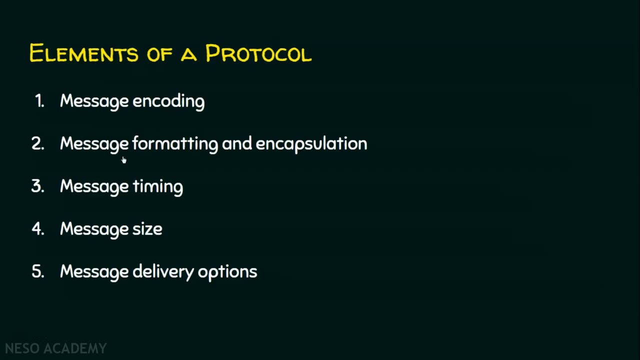 That should also be dealt in the protocols part. So a protocol defines message encoding, message formatting and encapsulation, message timing, message size and the delivery. That is what we exactly call as elements. The elements of protocol are message encoding, message formatting and encapsulation, message timing, message size and message delivery option. 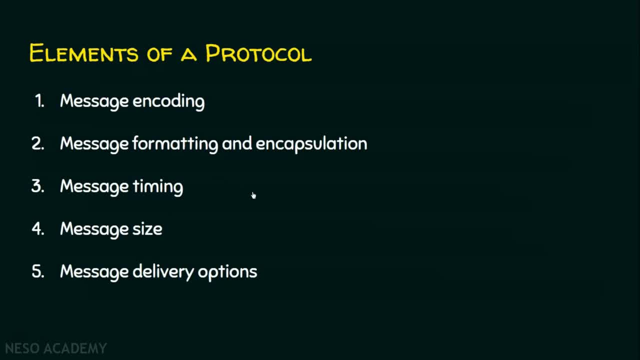 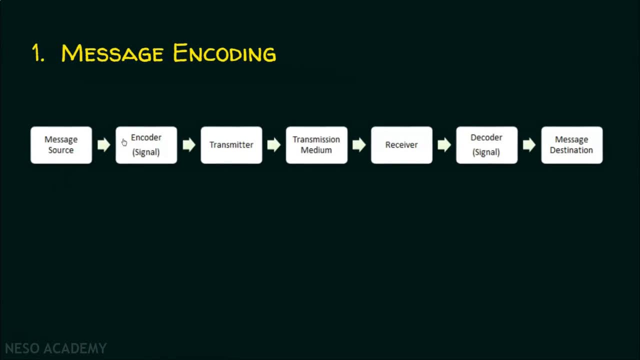 We shall see each of these elements in a detailed manner. Message encoding means the source, that is the source computer generates a message, it gives that message to the encoder in order to generate signals. Once the data is converted into signals, now it is given to the transmitter for transmission. You may be getting confused why we need encoder here. Because we have two kinds of transmission medium. 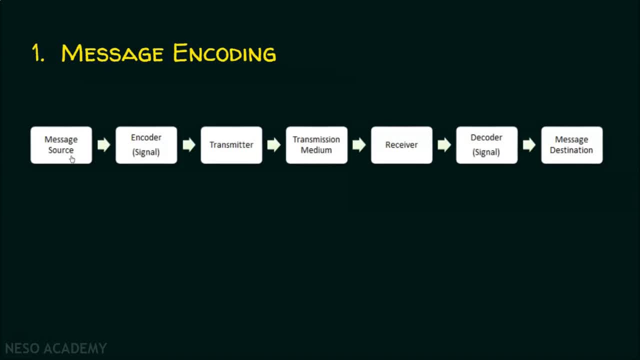 One is a wired medium, another one is a wireless medium. The source have to understand to which medium it is connected to. 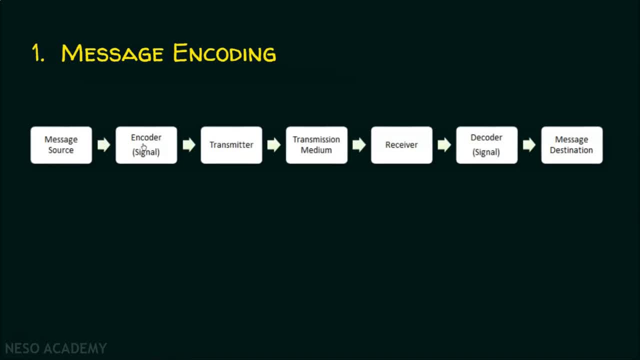 If it is a wired medium, the data have to be converted into signals in order to facilitate the data transmission on a wired medium. 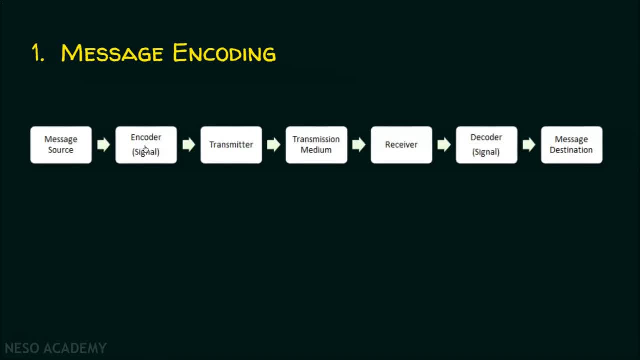 If it is a wireless medium, the sender have to encode the data in the form of waves. Because this is a wireless medium, we can't send signals, we have to send waves. 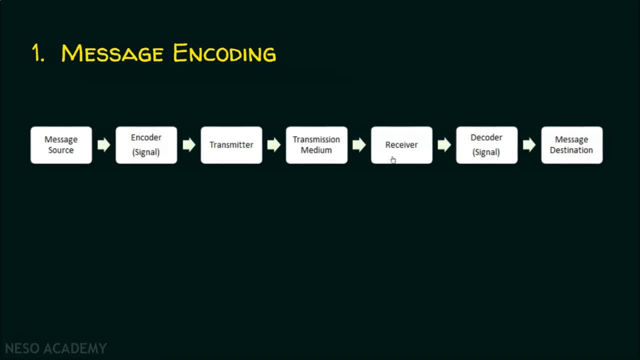 And once the data is sent through the transmission medium, the receiver receives the data and decodes it. Decoding means understanding it. After understanding it, 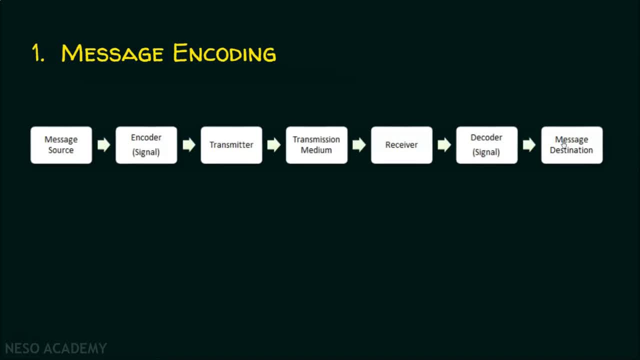 it means the message has reached the destination. This is what message encoding is all about. 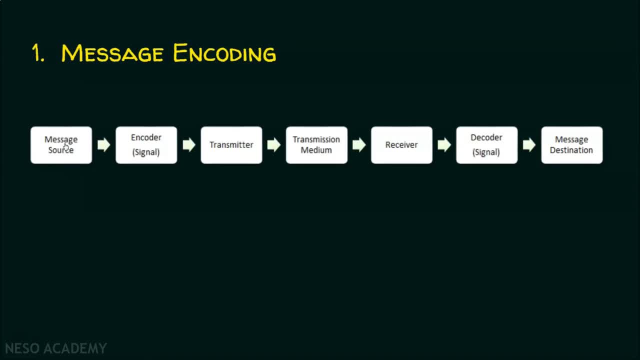 The sender sends the data, the sender creates the data and encodes the data. And finally, the transmitter sends the data through the transmission medium. 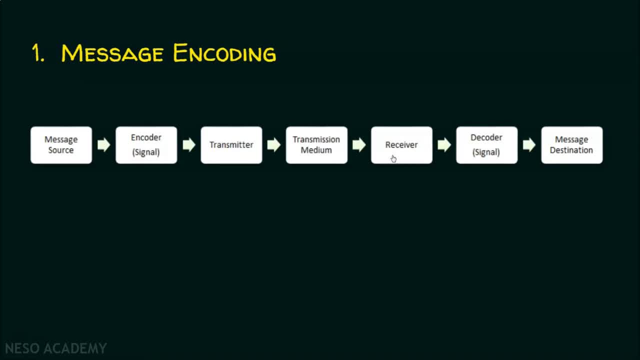 This transmission medium takes the data to the receiver. The receiver after receiving the data, it decodes the data and after proper decoding, it means the message has reached the destination. 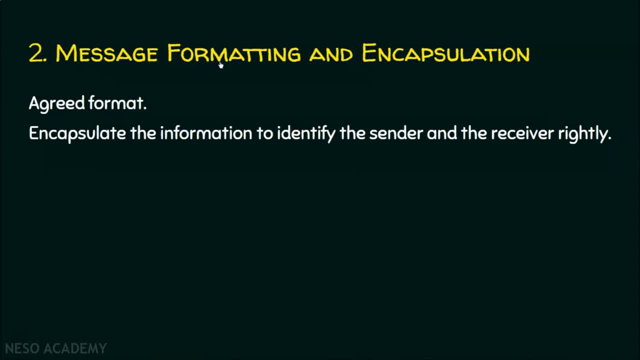 We shall see the second element of the protocol, that is the message formatting and encapsulation. Both sender and receiver must mutually agree upon certain formats, which we call as formatting. 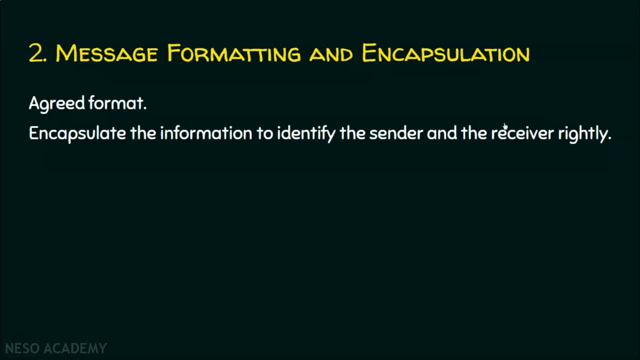 At the same time, when the receiver receives some data, it should identify who has sent this data. We are going to add some information with the data in order to identify the sender and the receiver. So we are not going to just send data as such, we are going to encapsulate certain things like the source information, and the destination information with the data. So that the right sender and the receivers are identified. And the third element in the protocol part is message sizing. 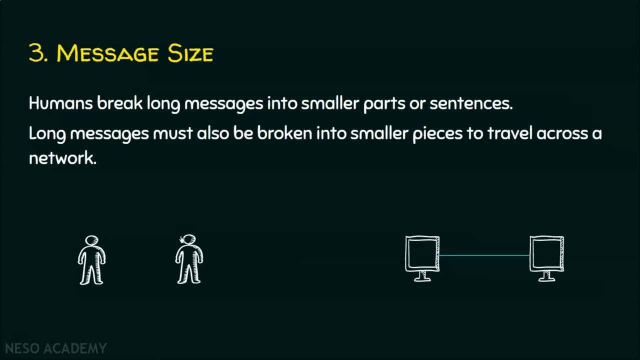 If there is a very big message to be communicated to the destination, 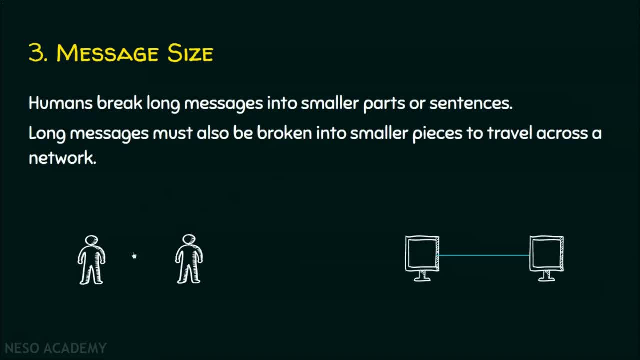 human breaks the message into smaller parts or sentences. 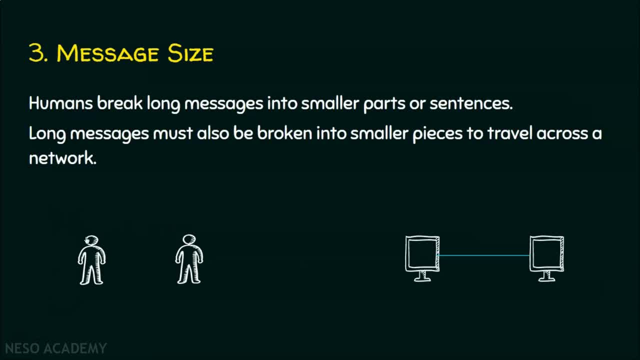 Say if this guy has a very big content to be sent. So what he does? 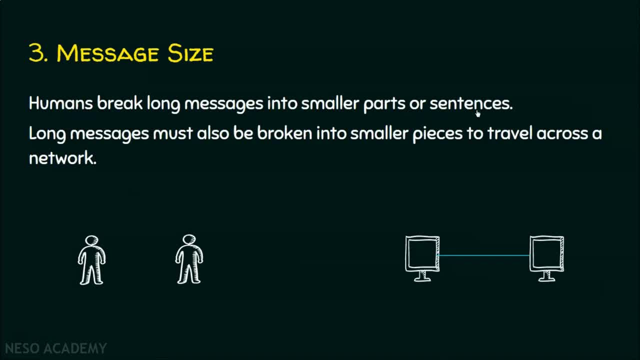 He breaks the message into smaller parts or sentences. 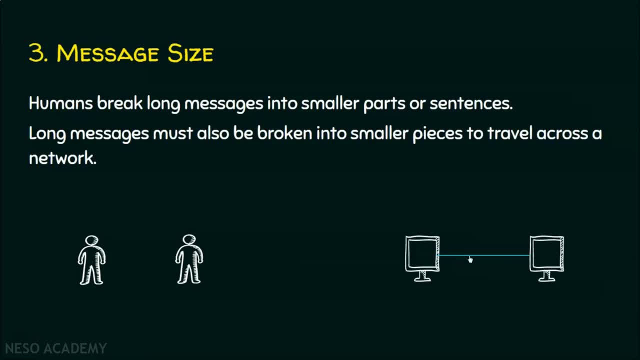 Likewise, our computer should also do that. If the capacity of the link is very small, but the data to be transmitted is very big, this computer should break this big message into smaller units, which this transmission medium can handle. 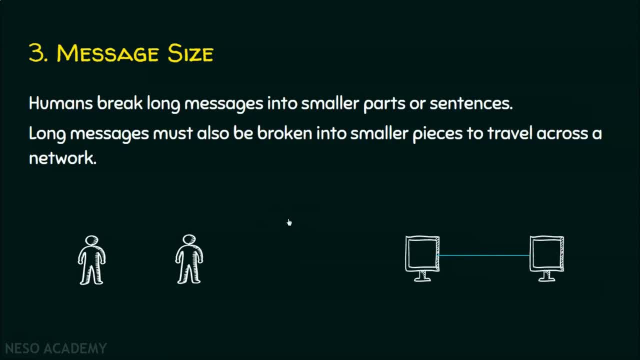 This is what message sizing. And this is one of the thing a protocol should do. 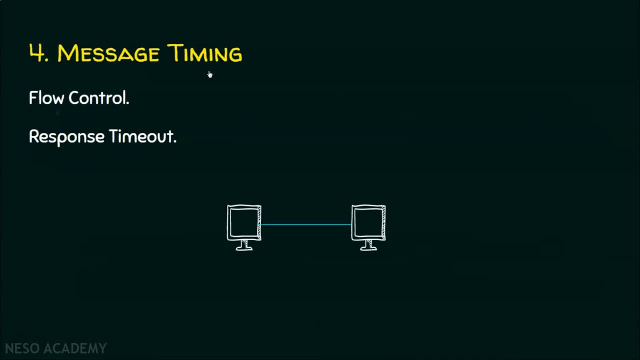 And message timing is the fourth element of protocols. And message timing deals with flow control and response timeout. 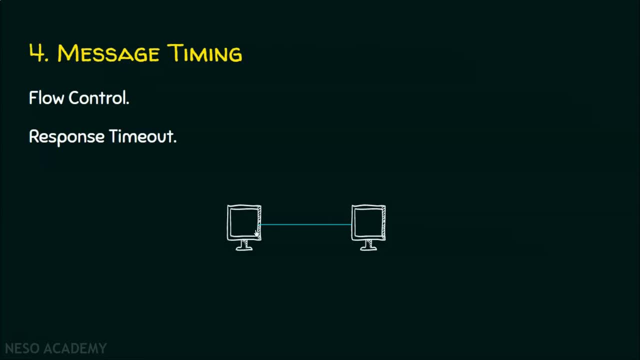 Let's first talk about flow control. Let's assume this guy is very fast, and the receiver is slow. Since the sender is very fast, it can send data at high speed. 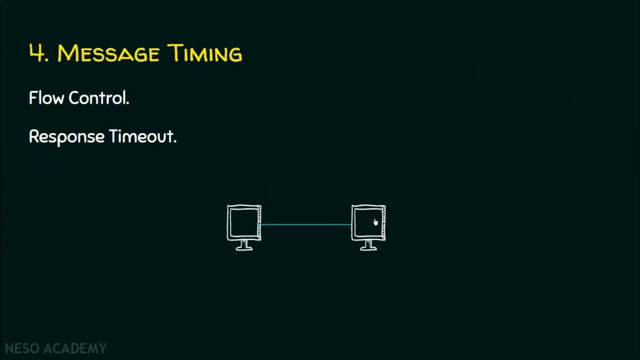 What about the receiver? He can't handle that speed. 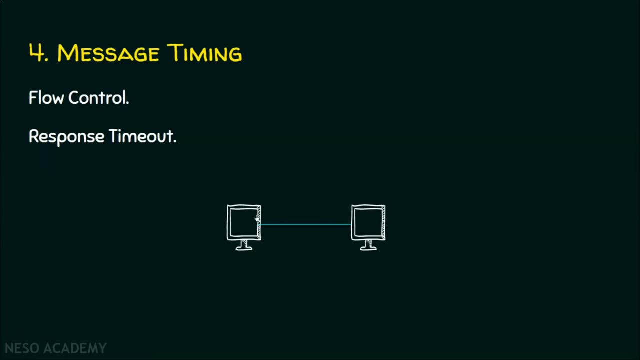 If there is no flow control mechanism, he can keep on sending data, but he cannot receive that data. 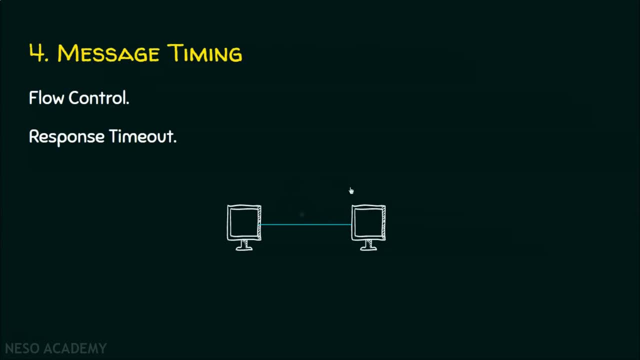 So the entire communication will become useless. It is the responsibility of the protocol to provide flow control mechanism. 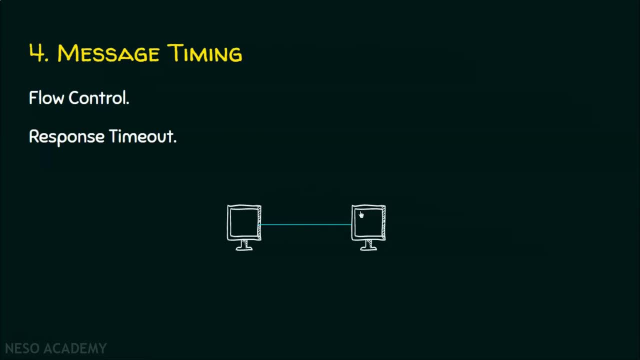 At the same time, if the sender is sending some data, and the receiver has to acknowledge the data, when the acknowledgement is sent back to the sender, the sender can understand that the data is received by the destination. 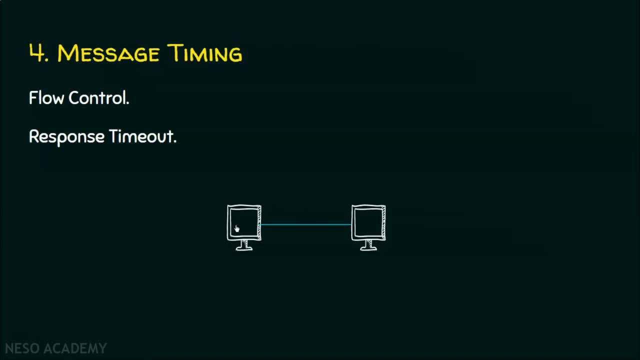 If the acknowledgement is not received, the sender have to wait for a certain period of time. After the expiry of the time, the sender will retransmit the same, 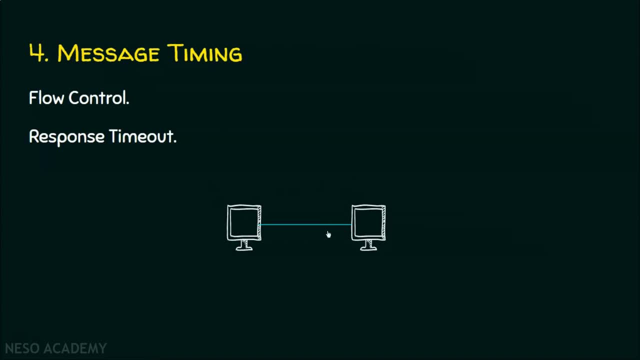 so that we can ensure guaranteed delivery. And it is the responsibility of the protocol to tell how much time this computer should wait for an acknowledgement. 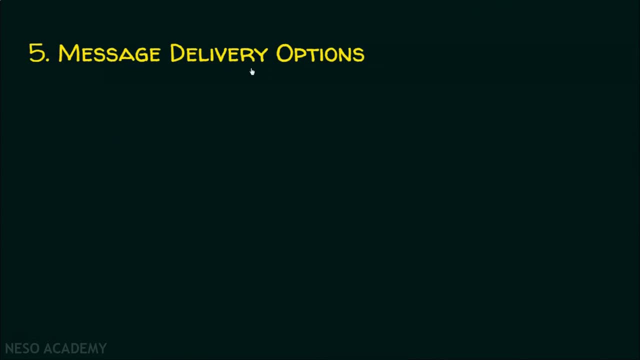 And we have the last element of the protocol, the message delivery options. There are three delivery options. 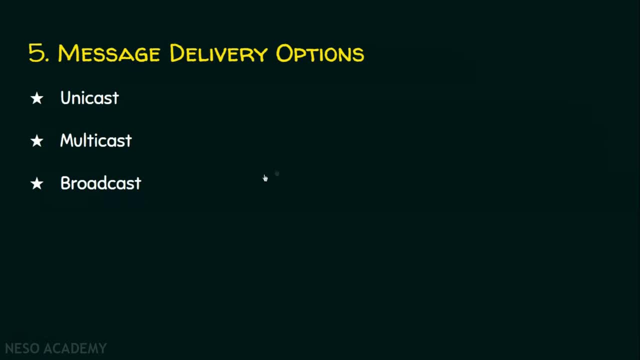 One unicast, two multicast, three broadcast. 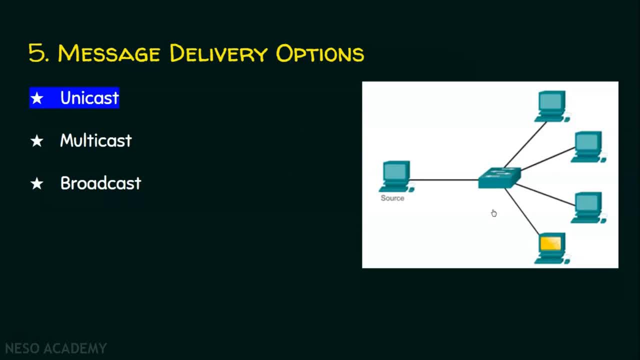 Unicasting means one sender and one receiver. It means this sender is going to send data to exactly one receiver in the network. 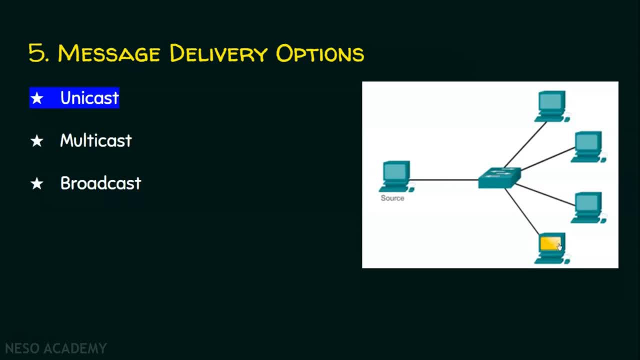 If the sender is sending the data to exactly one destination, it is called as unicasting. If the sender sends the data to set of receivers, but not to all, then this is multicasting. 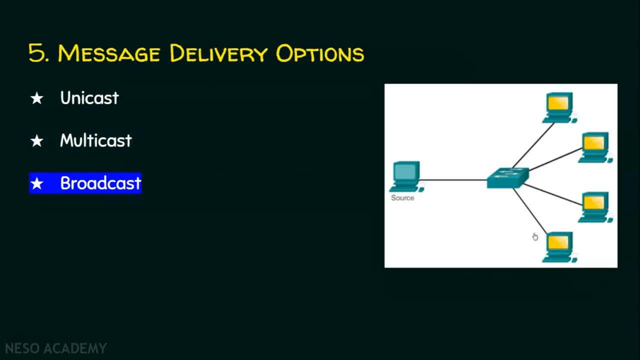 Broadcasting means, the sender sends the data to all the participants in the network. And that's it guys. 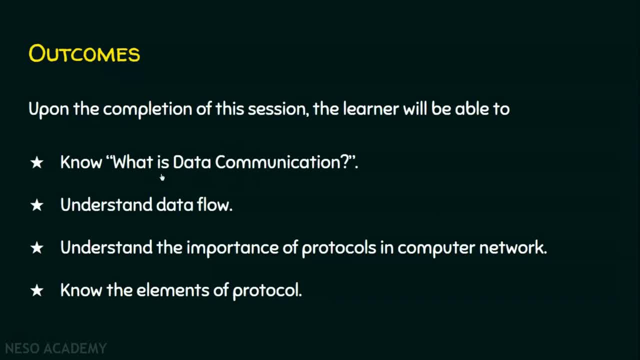 Now we shall just recapture what we have seen today. We have seen what is data communication. That is the exchange of data between nodes. And we have also seen what is data flow. And we have seen the three data flows, simplex, half-duplex and full-duplex. 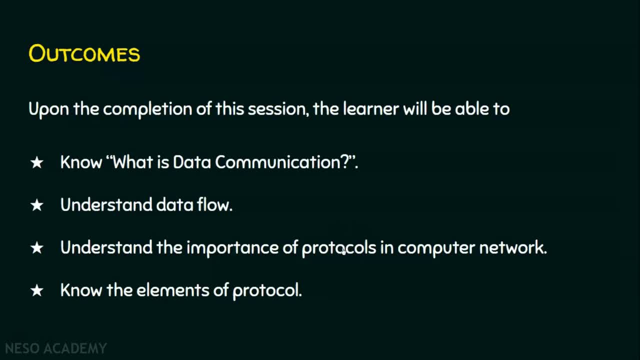 We have also seen the role of protocols in computer networks. Not only in computer networks, even in real time, 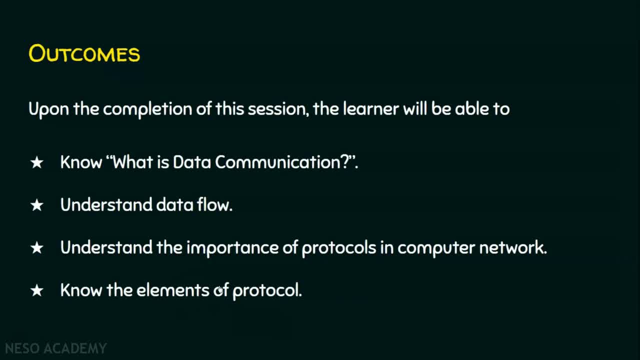 protocols has a very important role to play with. And we have also seen what are the elements of protocols. 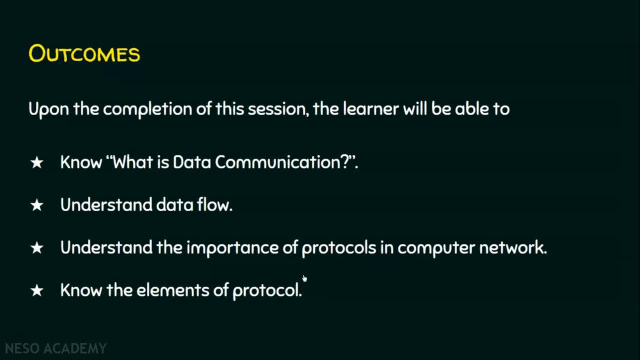 There are five elements of protocols. Message encoding, message formatting and encapsulation, message size, message timing and finally the delivery options. I hope this session is informative. Thank you all.